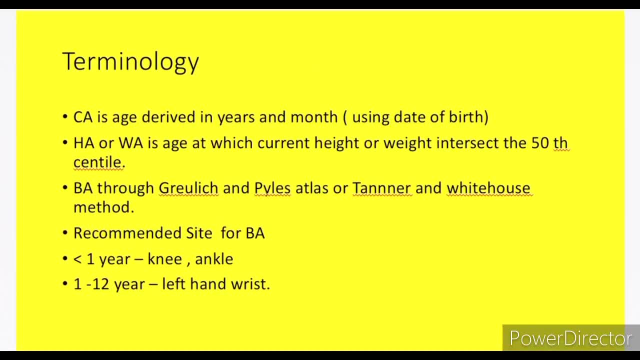 So before plotting growth chart, we must know some terminology. What is chronological age? Chronological age is defined as chronological age By simply using date of birth. we can tell this is the chronological age- It is in year or month- simply by using date of birth. 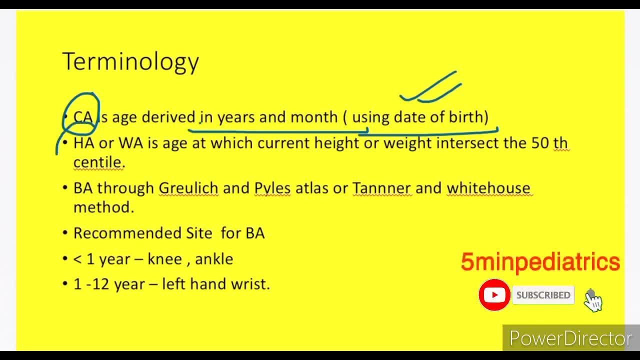 Now, what is chronological age? Next we have height age or weight age. It is defined the age at which current height or weight intersect at 50th centile. Better you will understand when we will draw in growth chart. And bone age is estimated through Goudlitz and Piles, Atlas or Tanner and White. 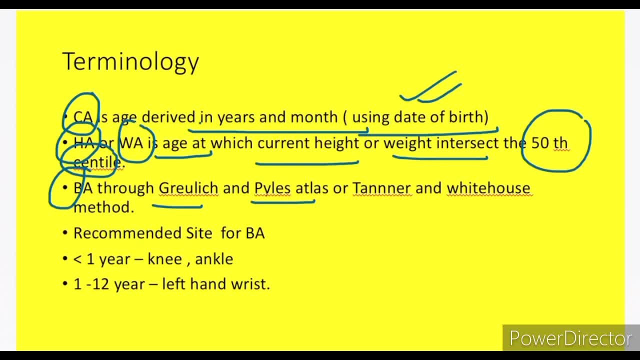 House method. So site for bone age, we took X-ray of knee or ankle joint if the age is less than 1 year And from 1 to 12 year, generally non-dominant hand, that is, left hand wrist joint. So another term we have: Mid-parental height. Mid-parental height is mother height plus father height, divided by 2 plus minus 6.5. This is mid-parental height. If the child is boy, just add 6.5.. 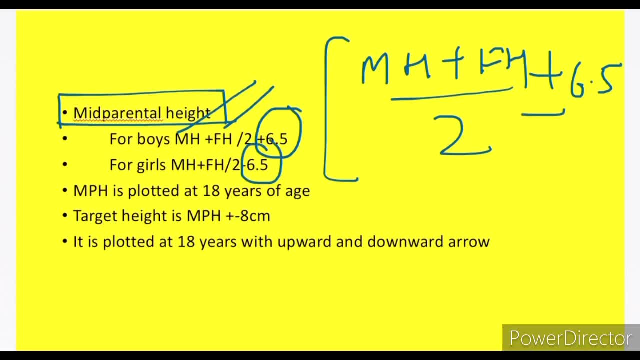 If the child is girl, subtract minus 6.5.. Mid-parental height is plotted on extreme of the growth chart at the 18 year of age And one other term we have target height. Target height is mid-parental height plus minus 8 centimeter. 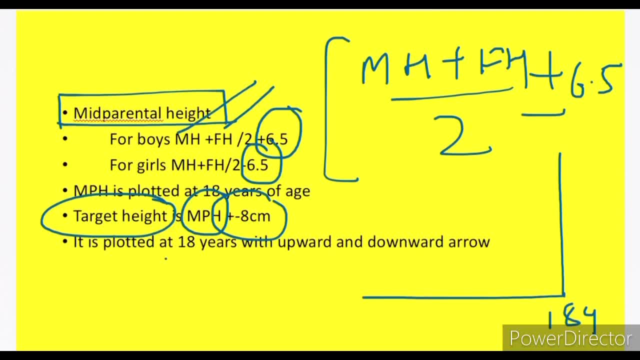 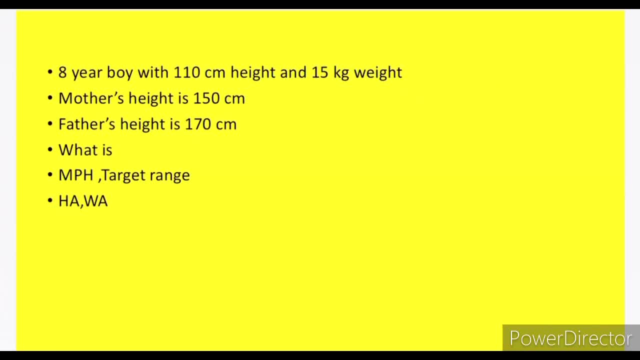 And it is plotted at 18 year with upward and downward arrow. Okay, Better you will understand with question. So we have 8 year boy, Okay, With height of 110 centimeter and weight of 15 kg. Mother height is 150 centimeter and father is 170 meter. 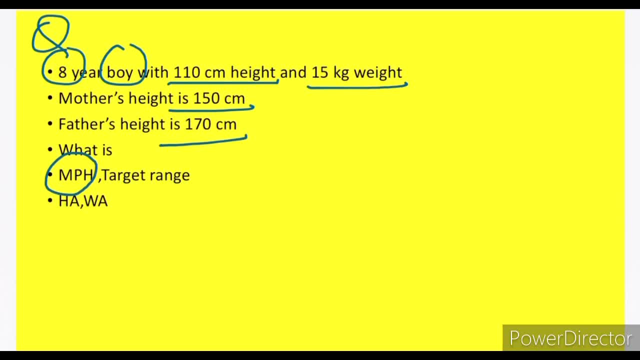 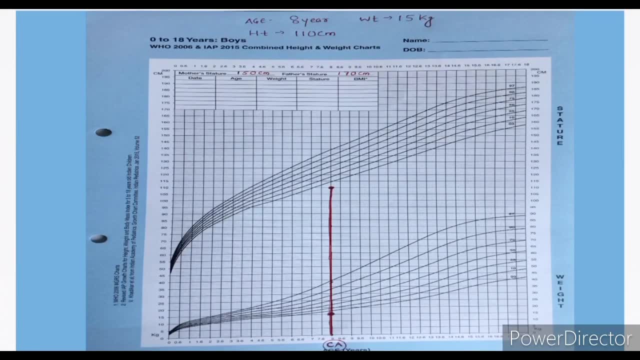 So now we will calculate mid-parental height target range, height age or weight age. So this is the growth chart for boys B, for boys B for blue color And for girl we have pink color. Okay, So this is growth chart IAP plus WHO, both combined growth chart up to 18 year of age. 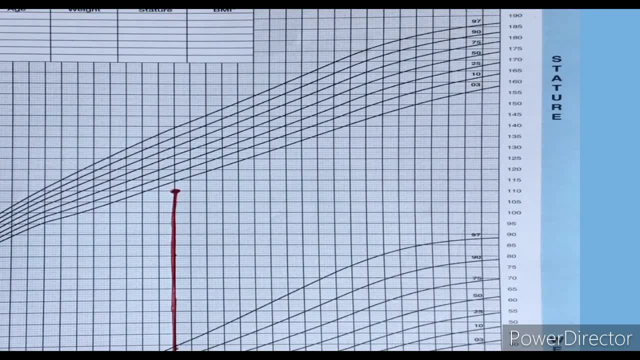 On x-axis we have age and on y-axis we have weight and height. So first of all we will draw chronological age. The height of the child is 110 centimeter and weight is 15 kg. Okay, So here we have 8 year with 15 kg. 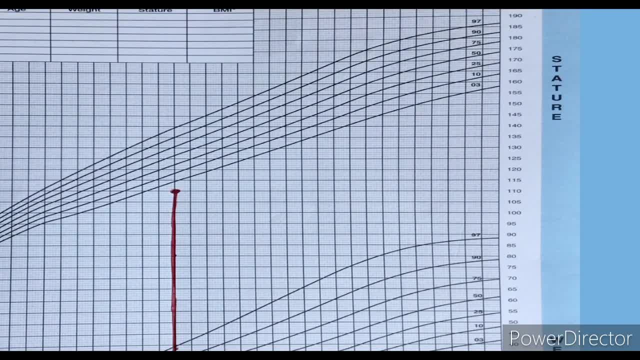 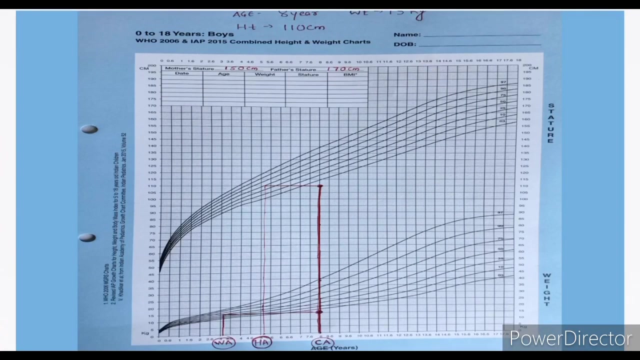 This is chronological. This is chronological age. Weight is here and height is 110 centimeter and we draw at 8 year of age. This is chronological age. Now we will draw. what is height, age or weight age? Okay, Already told that the age. this is the chronological age. 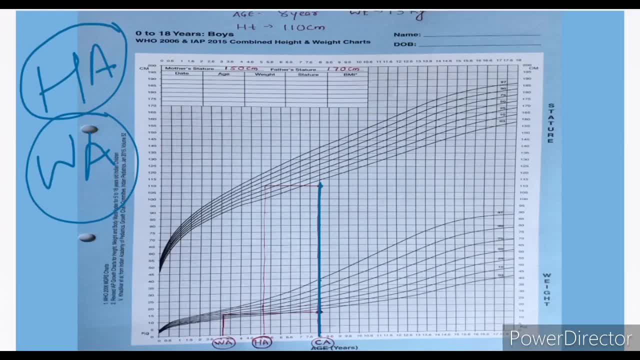 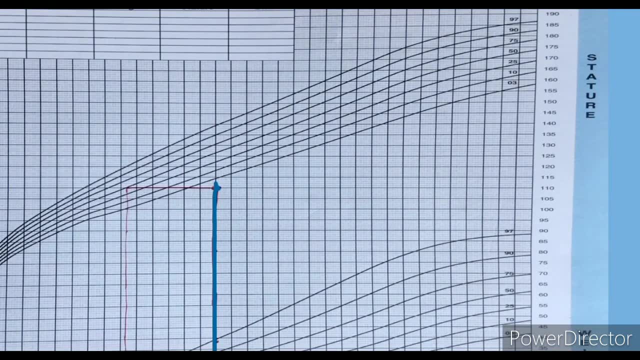 For height age. look for the 50th centile by going backward. So this here we have 3rd, 10th, 25th and 50th. So going backward, this is the 50th centile. 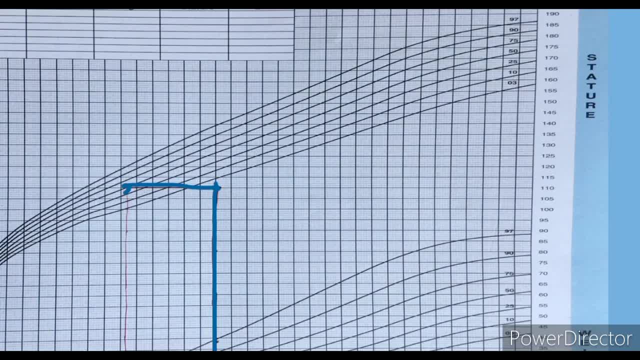 Here it intersects. From this point draw a perpendicular line downward. It comes in between 5 to 5 and 6 here. So this is the height age. Similarly we can draw weight age. This is the 15 kg. 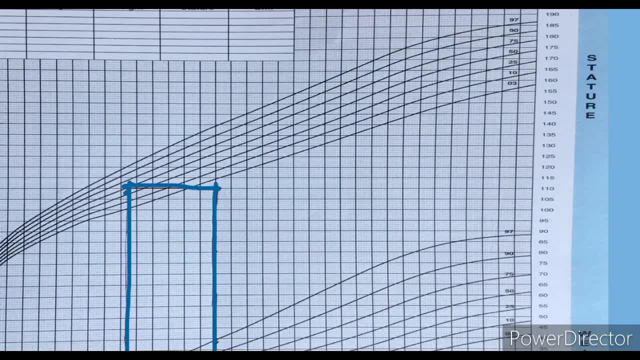 15 kg child and look for the 50th centile going backward and it intersects the 50th centile here in between 3 and 3.6 here. So this is weight age. We can easily draw height, age and weight age by this method. 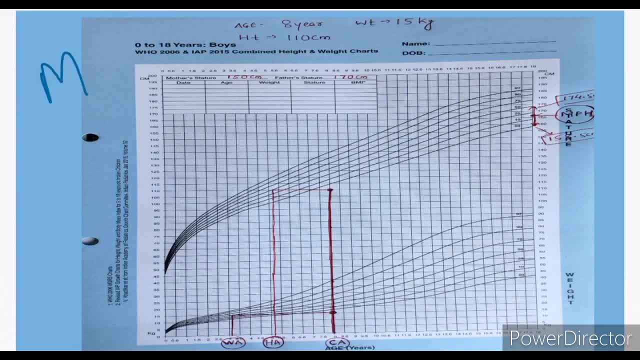 Now we will calculate mid-parental height. Okay, And what is target range For mid-parental height? already told that it is average of mother height and father height. Average of mother and father height is 150 centimeter plus 170 centimeter divided by 2.. 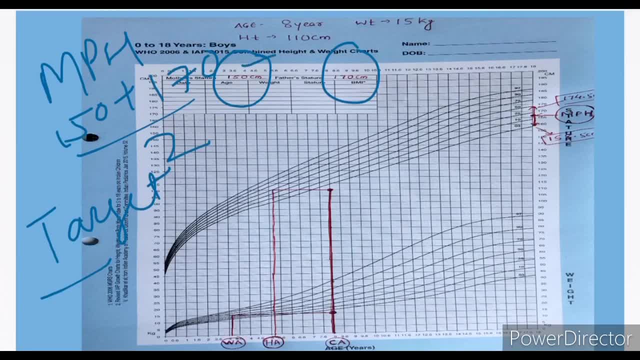 The case is wise. So we add 6.5.. So we have 166.2.. 5 is mid-parental height, and mid-parental height is drawn on extreme at the 18 year of age, And if we enlarge the curve here we have 166 centimeter here. 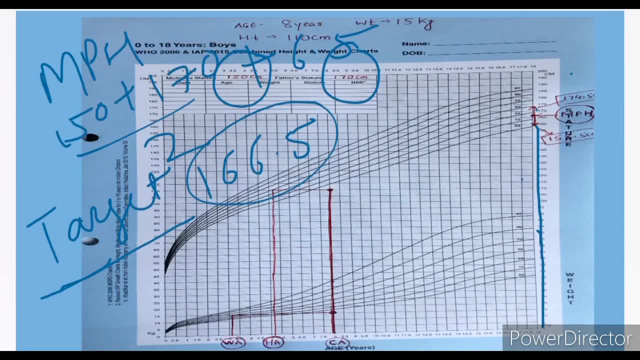 And if we want to draw target height, we again add plus minus 8 centimeter. This is the target range. Target 174 centimeter. and downward and upward we have downward 158.5 centimeter. So we can easily plot a growth chart by in this way. 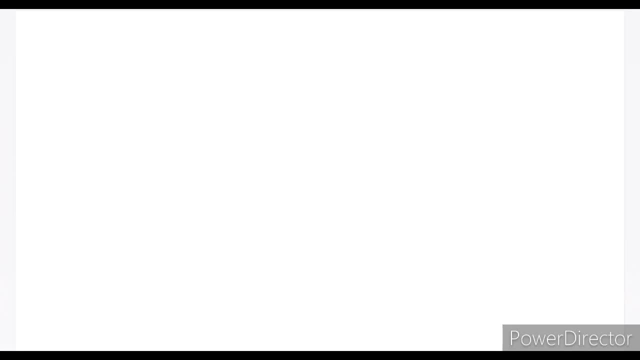 Now one question is frequently asked in DNV OSCE, question in the form of match, the following, or mostly in the match, the following: Okay, So in case of short stature we can easily minimize differential, Suppose we have growth velocity. 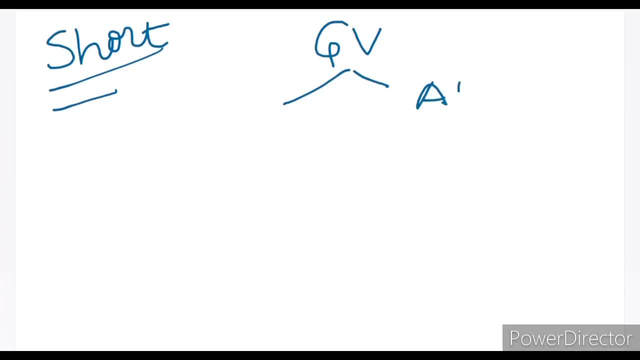 We have growth velocity, either abnormal and other we have normal. If we have normal growth velocity, we look for if chronological age is equals to bone age. Other condition: we have chronological age more than bone age And if chronological age is equals to bone age, we have familial short stature.